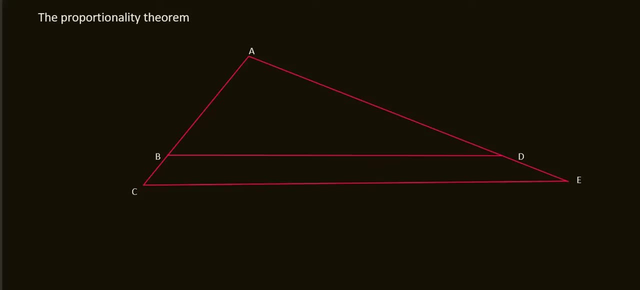 In grade 12 we start something called the proportionality theorem and it has to do with triangles. So whenever you have a triangle where you have two parallel lines- so let's say over here these two lines are parallel- then you can say the following: You could say that AB. 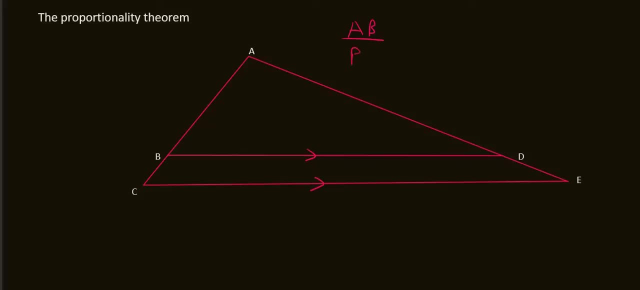 over BC. so see what I've done there. I've chosen that one, and then I chose that one. Well, that's going to be the exact same as AD over DE. So I'm not saying that the length of AB is the same as AD. You can clearly see that these two lengths are not the same. 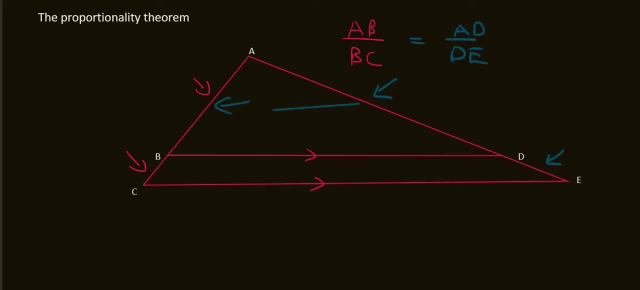 but it is the ratio that stays the same, And I could choose other combinations. I could say AB, so that's this one, over the whole length from A to C. Then on the other side, I would choose the same length from A to C. So I could choose the same length from A to C. 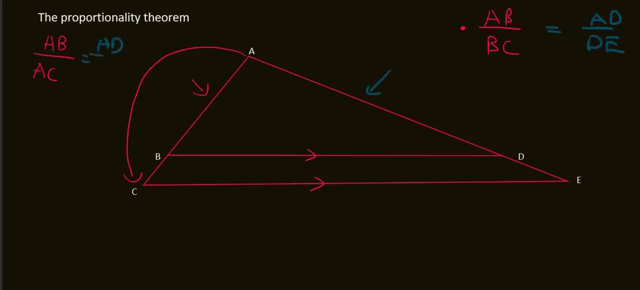 I could choose AD and then I'd have to choose the whole length of AE, And in fact you can choose any combination that you like. You could, for example, start with BC and then make that go over AB, for example. Then, as long as on the other side, you match it. So BC matches with DE and 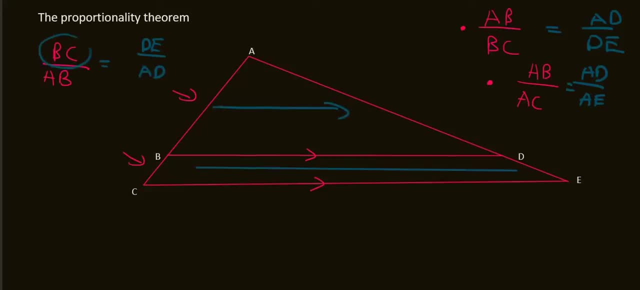 AB matches with AD And over here. whether you write BC or CB, that doesn't really matter. So you can choose any two on the left-hand side and make it equal to the other two on the right-hand side, as long as the order stays the. 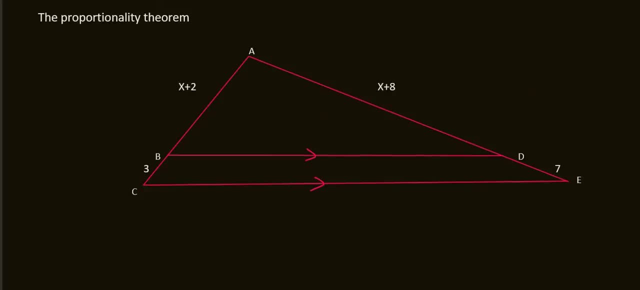 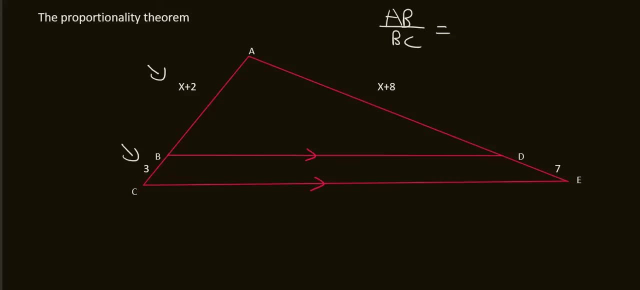 divided by this one must be equal to. Now you match it. So on that side it's going to be AD over DE. Now what would your reasoning be? Well, I've seen two different types of reasons that different students use. The more common one is: people say prop theorem because that stands for.